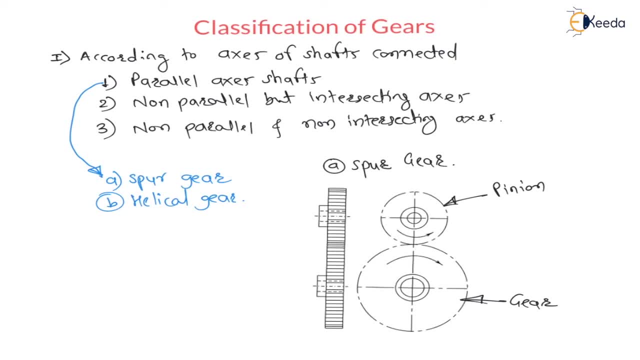 and this is the front view. now, in front view we can say that if gear is rotating in clockwise direction and for external contact, the pinion will rotate in anticlockwise direction. right, because the common point here, this common point, is trying to move in forward direction with 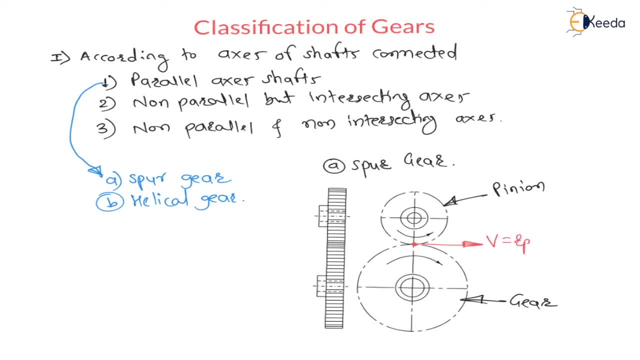 constant velocity, which is nothing but radius of pinion, angular velocity of pinion, which is not equal to radius of gear, into angular velocity of gear. that already we have seen in introductory lecture. right, as this common point is moving towards right. therefore, the gear must rotate. 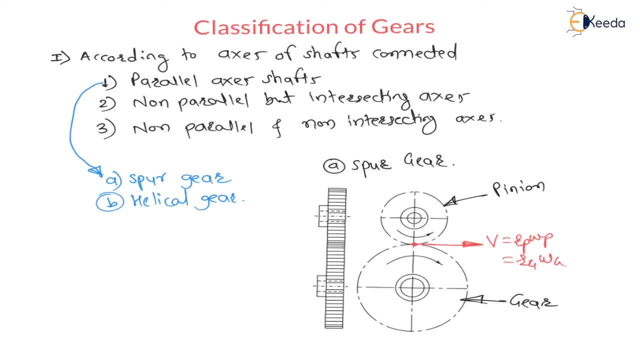 in clockwise direction, And pinion must rotate in anticlockwise direction and it is called rolling motion. they are rotating, therefore it is called rolling motion, and we can see the teeths are cut parallel to the excesses. now let us say in another view: see, this is the axis of pinion, this is the axis of pinion, and here 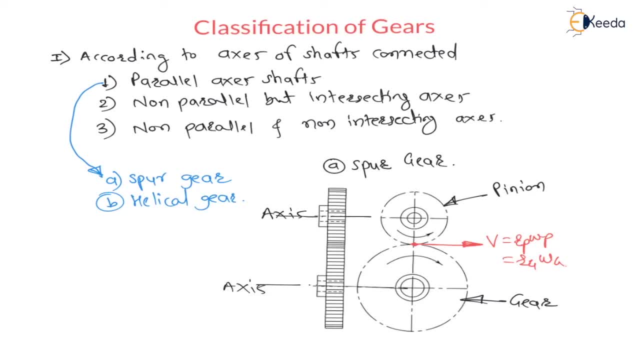 it is a axis of gear, axis of gear and here on these there are, teeths are cut. these are the teeths cut and teeths are parallel to the excesses. teeths are parallel to the excesses and straight means we can say. second point which is very important is teeths are straight and parallel. 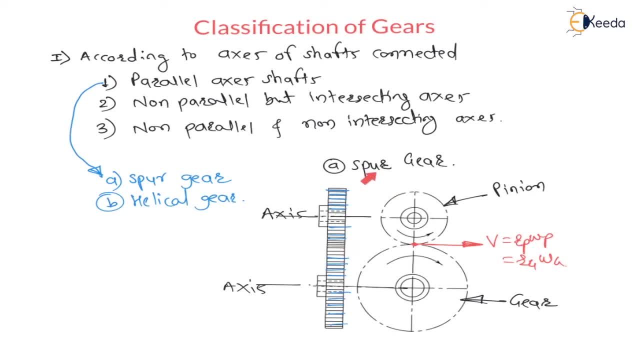 to the excesses. generally the use of spur gear is limited. they are not used because there is a instantaneous engagement and disengagement. in spur gear there is instantaneous engagement and disengagement. we can say this is the easiest way to find out the difference between these two points. 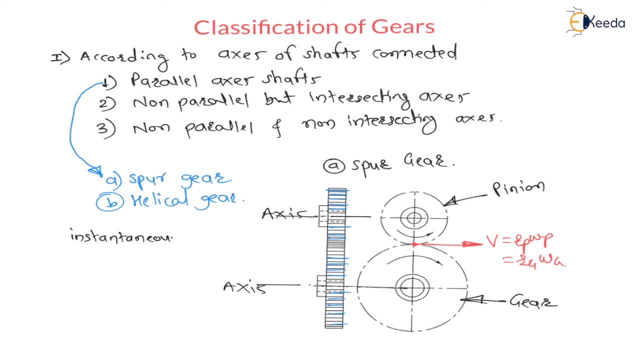 say instantaneous, or we can say sudden, sudden engagement and disengagement and this engagement right. because of this, because of sudden engagement and this disengagement, there are impact stresses on the tooth, impact stresses on the tooth and, because of this, tooth fail earlier than other gears. therefore, because of these advantages, there is sudden engagement. therefore there are impact. 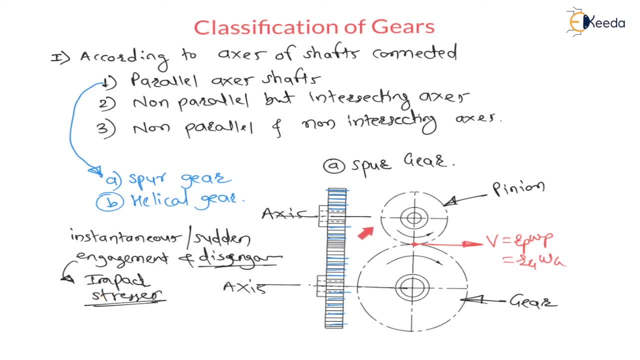 stresses. therefore, generally, spur gears are avoided, but for very low power transmission, at very low speed, spur gears are preferred. note down the statement: at very low power transmission, at very low speed, spur gears are preferred. for example, watches: in watches, spur gears are preferred. now, if you have a hand watch, right, then you can. if, if you open this watch, in this watch, all the gears. 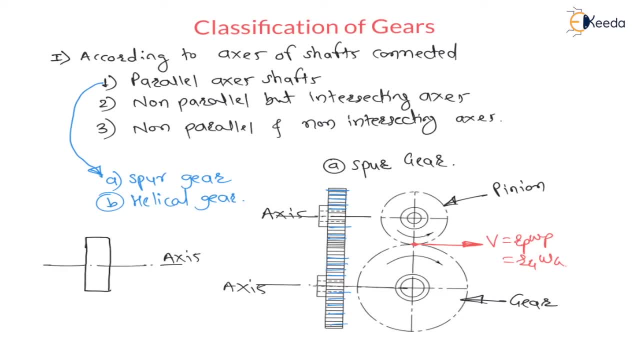 are spur gears. now here for axis, the teeth are cut parallel like this. the teeth are cut parallel like this, and whenever load acting on this gear, the load is perpendicular to the teeth. this is a load. therefore, we can say there is a load along radial direction only it is called radial load. 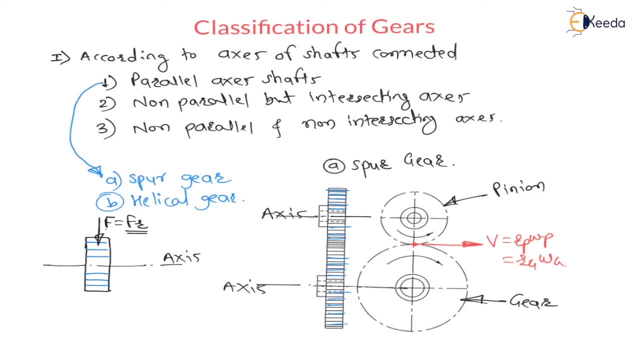 only it is called radial load and the component of this total load will not come along axial and the component of this total load will not come along axial direction. therefore, axial load in case direction, therefore axial load in case of spur gear is zero. this is main advantage here. this is main 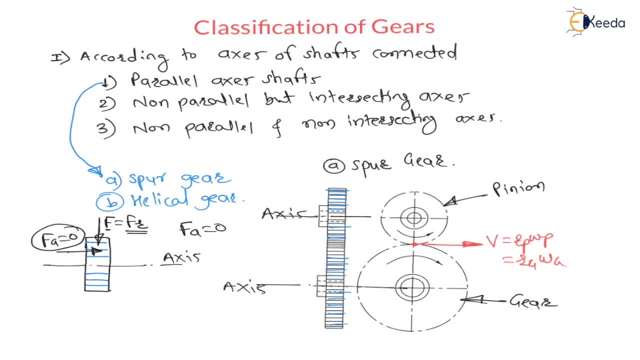 of spur gear is zero. this is main advantage here. this is main advantage that that is axial load. which advantage that that is axial load, which is called thrust. this is also called axial thrust or thrust is called thrust. this is also called axial thrust or thrust. in case of spur gear, thrust is zero. but 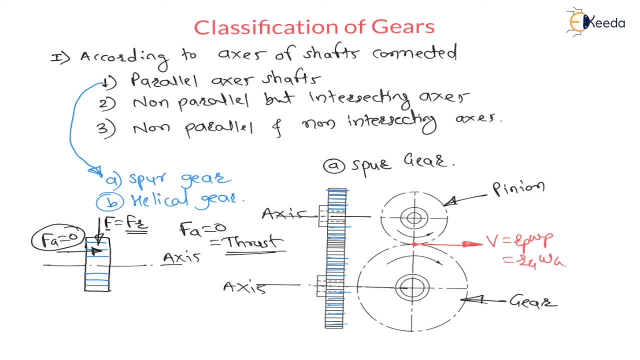 in case of spur gear, thrust is zero, but, yes, there is radial load because of contacting surfaces. there is, yes, there is radial load because of contacting surfaces. there is radial load because of contacting surfaces. there is radial load because of contact surfaces. hence, the main points regarding spur gear are the number one. 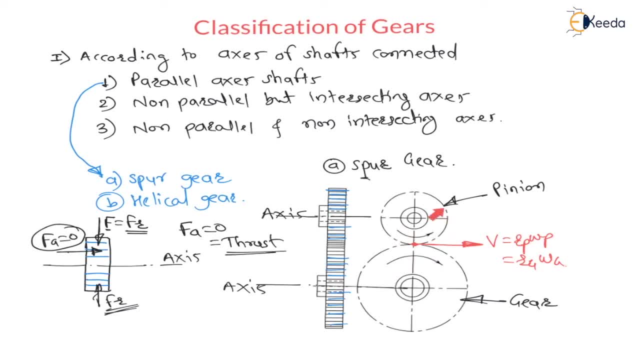 is there is a rolling motion, that is, one gear is rotating, other is also rotating and teeths are cut parallel and straight to the axis straight and parallel to the axis right. but the disadvantage is that there is a impact stresses because of sudden engagement and disengagement. there are 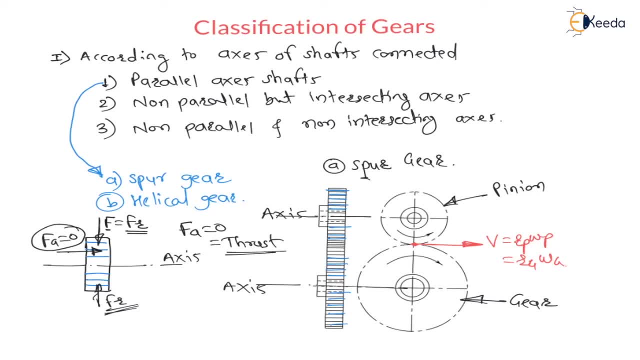 impact stresses. therefore the teeths fails easily. hence, generally the use of spur gear is avoided and the use is limited for very low power transmission and at very low speed, for example watches. and in case of spur gear there is only radial load and axial load is zero. 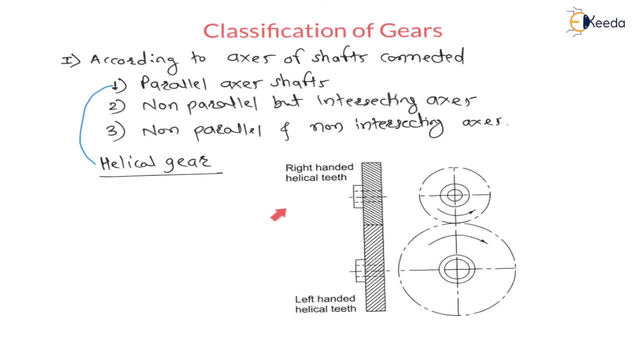 now to eliminate the problem of spur gear, that is, there is sudden engagement and disengagement because of this, there are impact stresses. now to eliminate this problem, helical gears are used and in case of helical gear, the teeths are cut at an angle with axis- see here for axis. if i consider, this is the axis, this is the axis, and 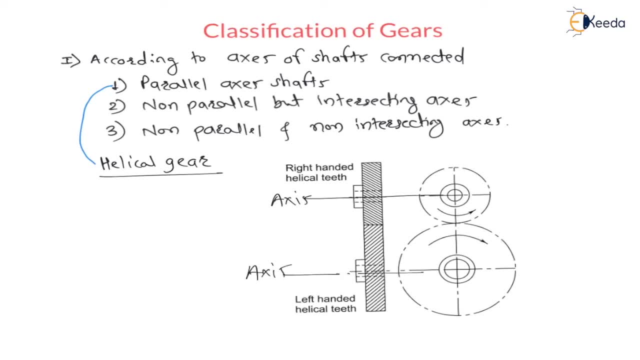 here this is the axis of gear, axis of gear and pinion. now the teeths are cut at an angle with axis. see the teeths are cut inclined to the axis. right here you can see the teeths are cut at an is circuited and inclination to the axis. in both view we can see now because of this inclination. 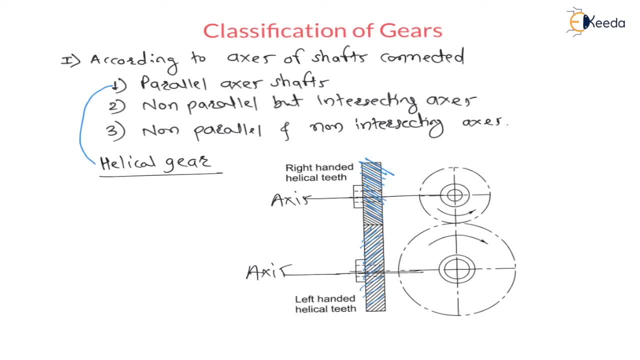 or helical angle. this is called helix angle. because of this helix angle, there is a gradual engagement and disengagement. because of this gradual engagement and disengagement, we can say gradual engagement as well as disengagement and because of this impact, stresses are eliminated. 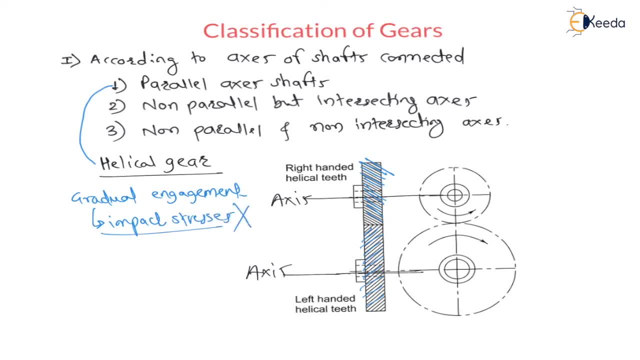 impact stresses are eliminated. there are no impact stresses and, my dear student, if you observe here carefully, there are. if i cut threads, if i cut right hand thread on the pinion, then compulsory for meshing we need left hand thread on the gear right see. here you can see. let us consider there is a pinion and gear in contact pl crocodile gear. this is the. 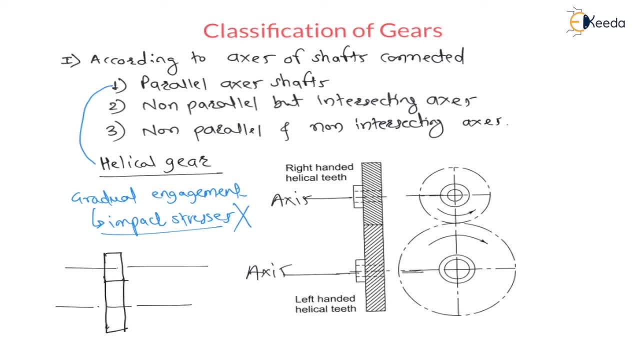 axis of theflix, which is the lateral axis of the sixth gear. there is a 놓 and longer one. it is smaller and long. it is a singular one is the Everpole and it is not straight on the axis as it moves. gear is the axis of pinion right now. if i cut right hand threads, that is going downward towards. 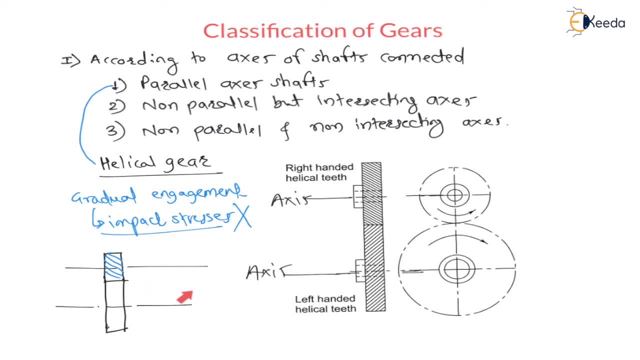 right. right hand thread means going downward towards right. right, these are, we can say: right hand thread on pinion, then on gear, compulsory the threads must be left hand, that is going downwards towards left. this is left hand thread on gear. then only there is meshing possible, right, you can see. 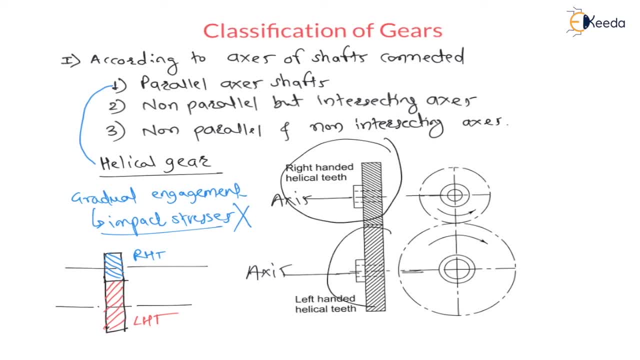 here on pinion right hand thread, on gear, there are left hand threads. now, because of this right hand and left hand thread, one problem arises, that is, the load acting on the thread is perpendicular like this: this is applied load and for this applied load we will get two components, that is: 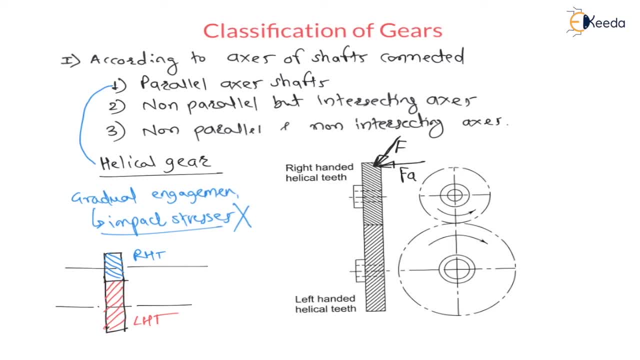 is one component along axial direction and one component along radial direction right, there will be a radial load also and there will be a axial load also. therefore, this axial load is called thrust means. in case of helical gear, there will be a radial load as well as there will be thrust. 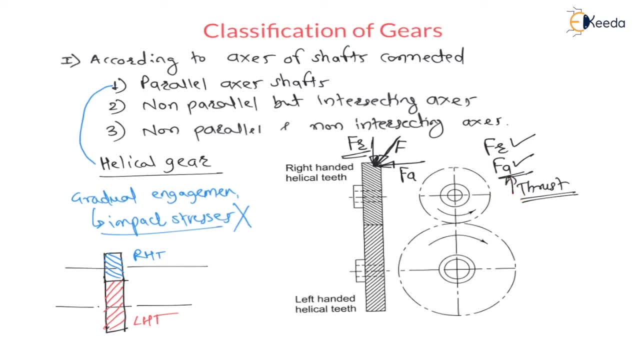 load and this is disadvantage of helical gear. now. so main points of helical gear are: the accesses are parallel. here you can find the accesses are parallel and teeths are cut straight and inclined to the accesses and the inclination is called helix angle or helical angle. and 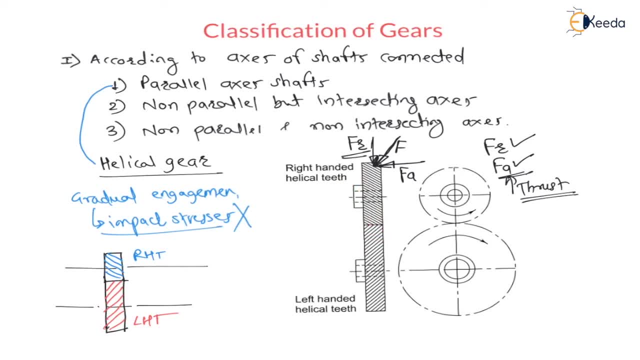 for here the main advantage we will get that because of this helical angle there will be a gradual engagement and disengagement and because of this impact, stresses are eliminated, completely eliminated, we can say. but on pinion, if there are right hand thread, you can see that the axis is parallel and the teeths are cut straight and inclined to the. 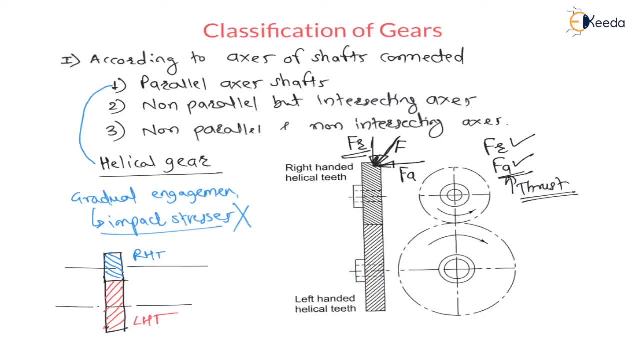 axis. then on gear compulsory, there must be left hand thread and vice versa, and because of this inclination of threads there will be a axial load as well as radial load. this is a disadvantage. now, to overcome this disadvantage of axial thrust or thrust, we are using double helical gear which 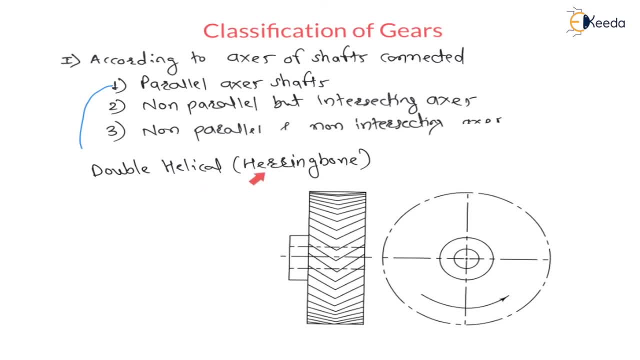 is also called herringbone gear. now here you can see double helical or herringbone gear. in case of double helical or herringbone gear, see the left hand, right hand thread are in contact like this right, left hand and right hand threads are. 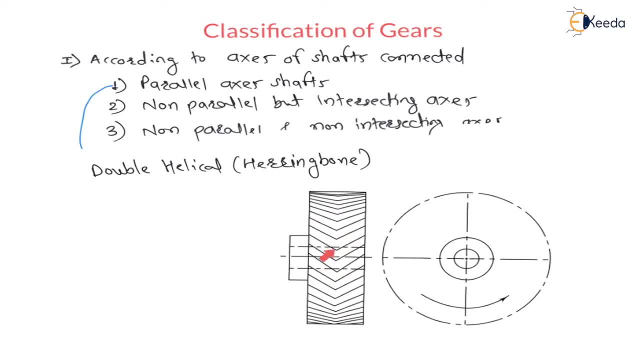 in contact like this: this is the only pinion, or let us say, only gear. here only one device is shown, not a assembly. right here you can see, these are the right hand threads and as well as left hand threads, means the gears are connected like this: let us say: this is one gear. 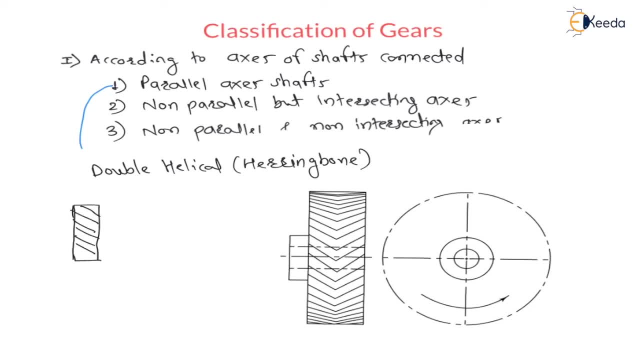 on which there are right hand threads now in contact with this. immediately there will be a another gear which will be having left hand thread. there will. they will be in contact right. this will be axis of them. now, because of this, the thrust problem is eliminated, that is, axial load problem. 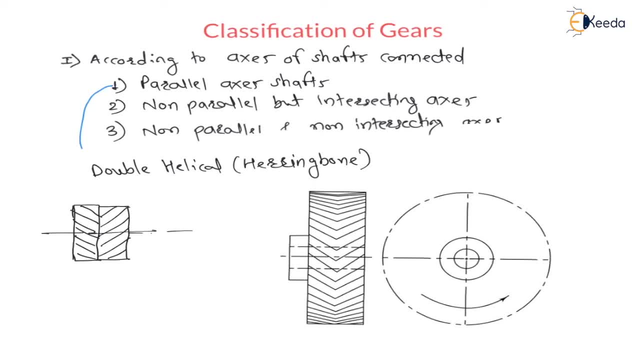 is eliminated. now see here, if i see axial load on the gears, see on this gear there will be a load like this: perpendicular to teeth. and on this gear the load will be like this: perpendicular to teeth. now consider any one load. for this load, let us say here there will be one radial component, fr, and there will be one. 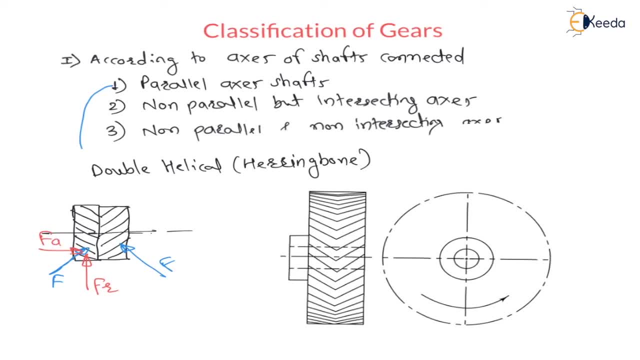 axial component, efa, and for another load, for another load, this, there will be one radial component, which is fr, and there will be one axial component, efa. right now, look at the diagram, my dear students. here the effect of axial load on one gear is cancelled by. 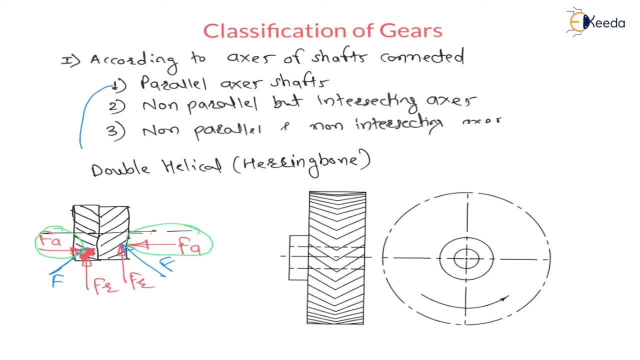 axial load on another gear. you can see here effect of axial load towards right on one gear is cancelled by effect of axial load on another gear towards left, and radial loads will get added. therefore, for double helical gear or herringbone gear, axial load is also present, radial load is. 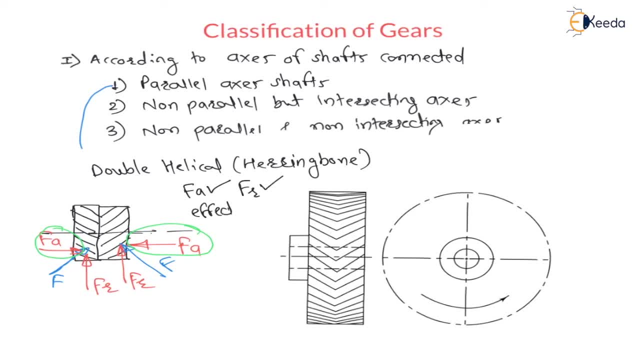 also present, but the effect of axial load, we can say effect of axial load- gets cancelled. each other gets cancelled each other. therefore, in case of double helical gear or herringbone gear, both loads are present but axial loads cancels each other. therefore the net axial load we can 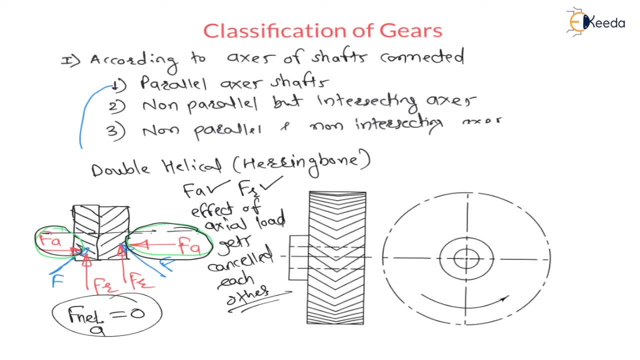 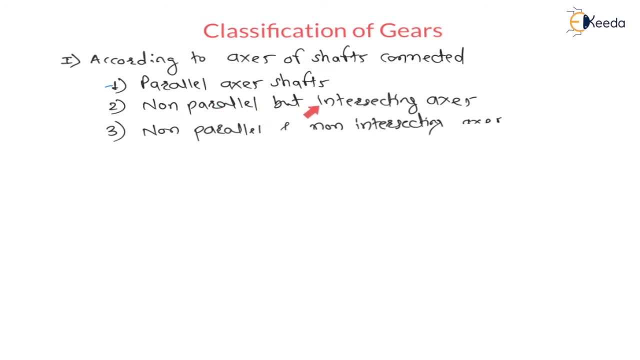 say the net axial load is zero. yes, there is a axial load, but the net axial load is zero. hence double helical gear is used to avoid the problem of thrust, which is called thrust now. the second type, according to axis of shaft, is non-parallel but intersecting axes in this. 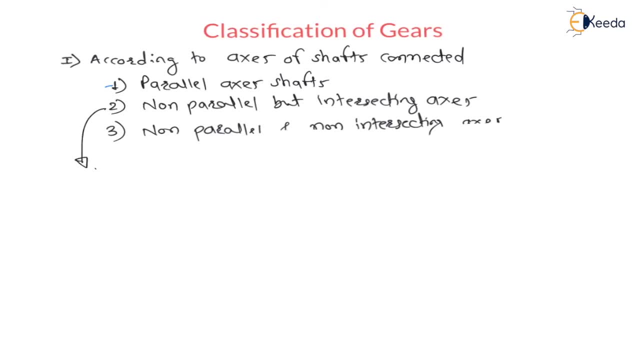 non-parallel but intersecting axes. there is a bivale gear- bivale gear again. this bivale gear is classified as straight bivale gear, straight bivale gear. another is zero bivale gear, zero bivale gear and by helical bivale gear. 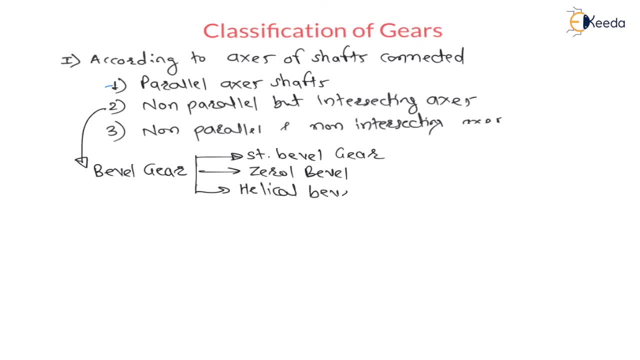 gear, helical bevel gear- right, These are the three classifications. Now, straight bevel gear and zero bevel gear are almost same. These are almost same. right, Now let us understand the bevel gear. Now, here for bevel gear, the axes are non-parallel. but as well as they are. 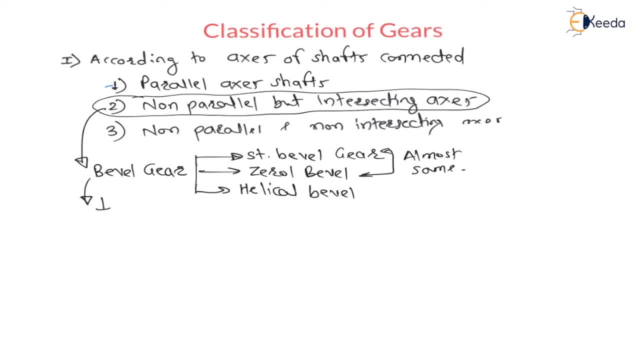 intersecting And generally the angle between axes is perpendicular. that is 90 degree, that is 90 degree. Generally 90 degree angle is used, But, yes, sometimes less than 90 or more than 90 is also used, but rarely right. So most of the time in bevel gear the power is. 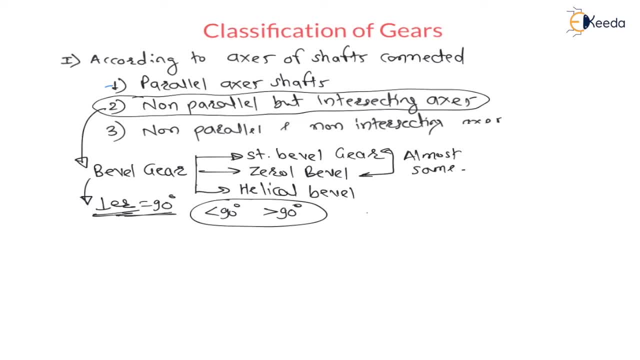 transmitted at 90 degree and the motion is rolling, motion only, pure rolling. they are rotating. Now, in case of bevel gear, in straight bevel gear and zero bevel gear, the teeths are straight and parallel to the axis of rotation. like spur gear. Like spur gear, the teeths are straight. 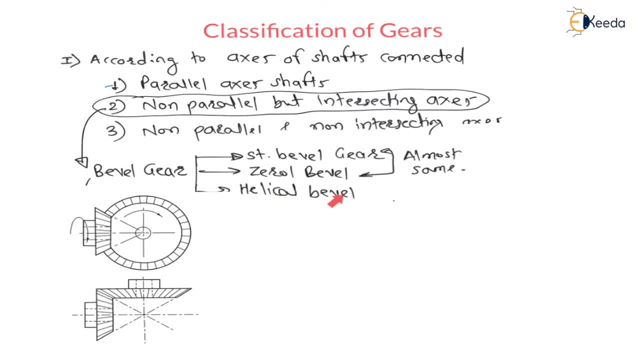 and parallel to the axis of rotation, And in case of helical gear the teeths are straight and inclined to the axis of rotation, like helical gear. But in spur gear and helical gear axes were parallel, But in case of bevel gear axes are non-parallel. 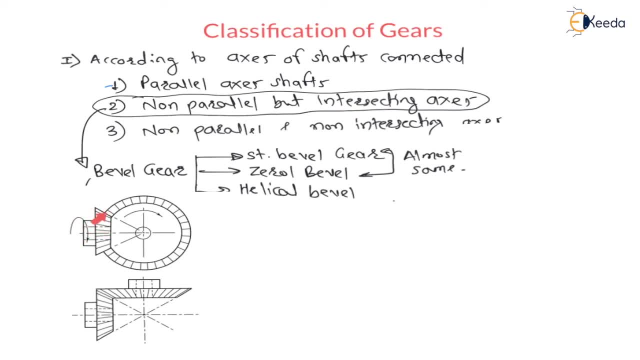 and intersecting. you can see here. see, there is one conical gear- this is a conical gear and another gear. right now their angle between them is 90 degree. see axis of one gear. see, this is a one axis and there is a another axis and angle between them is 90 degree. generally it is 90 degree, but 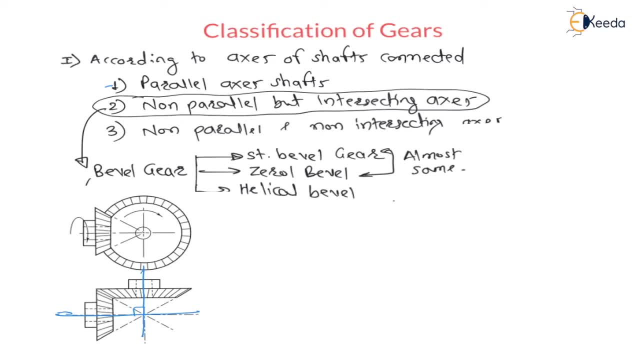 we can use more than 90 as well as less than 90, but generally it is 90 degree. therefore, whenever we want to transfer power at 90 degree or angular velocity at 90 degree, here it is a angular velocity rotating and here it is a angular velocity rotating means if you want to rotate the gears, 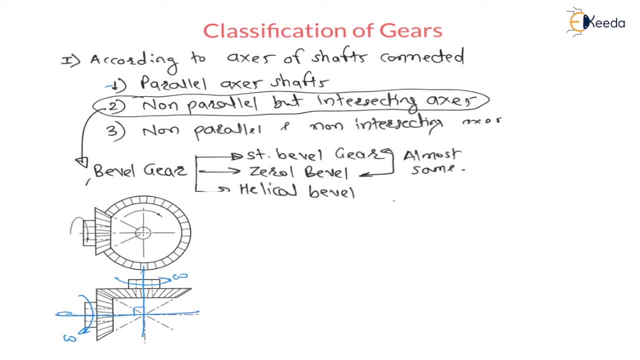 at 90 degree angle, then such type of arrangements are used. be well, gears are used now whenever angular velocity ratio, that is omega 1, let us say here, omega 1, omega 2, let us say, if i consider there is one gear like this, one gear, 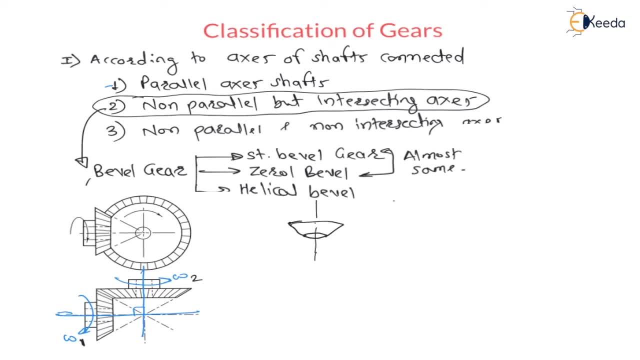 like this and this is axis. and there is another gear in contact with this like this and this will be axis. right now, let us say this is the first gear rotating with angular velocity omega 1. this is the second gear rotating with angular velocity omega 1, whenever this angular velocity ratio omega 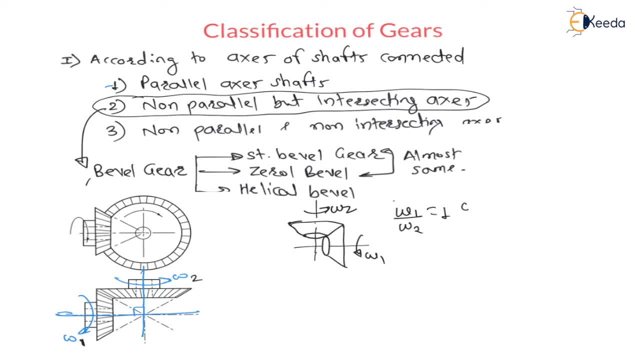 1 divided by omega 2 is equal to 1. that means angular velocity is not changing. here means it is neither speed reducing or neither speed increasing gear. it is only used to transfer power at 90 degree. such type of gear is called mitre gear. 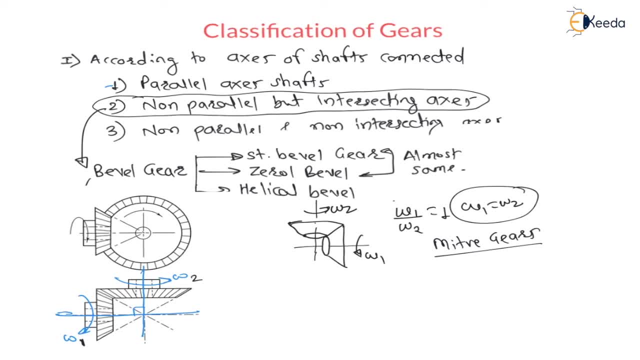 mitre gear. this is a mitre gear. right mitre gear is not increasing or decreasing the speed or angular velocity, it is only transferring the power at 90 degree. and in case of other omega 1 divided by omega 2 is constant, but not equal to 1 means it is speed reducing. 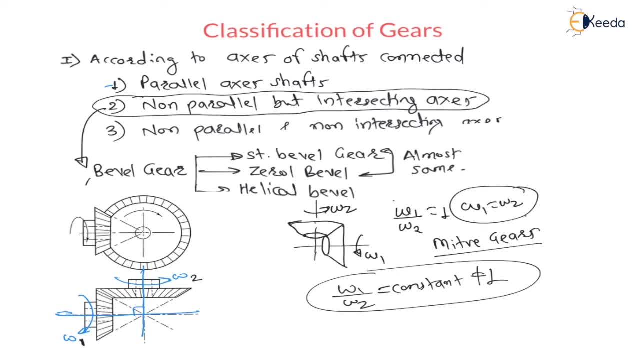 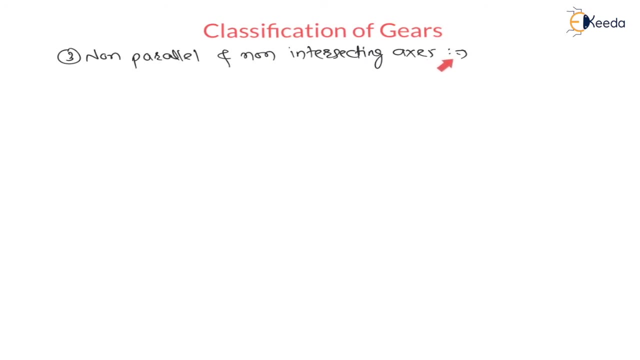 gear or speed increasing gear, bvl gear and in case of bvl gear, pure rolling motion is transferred. it means rotation is converted into rotation right, but at 90 degree. this is important. now, the 3rd type in the first classification is non-parallel and non-intersecting axes. in case of non-parallel, 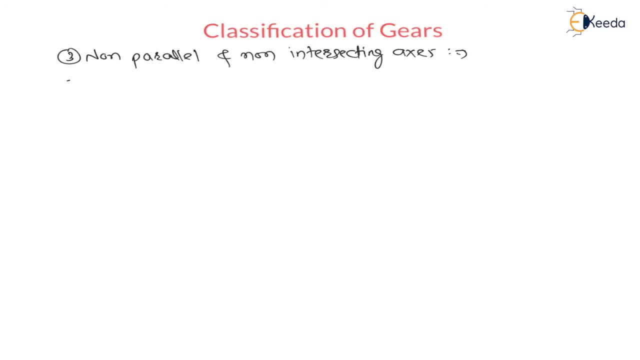 and non-intersecting axes, ess. pure rolling is impossible. we can say: pure rolling is impossible. possible means not possible. But yes, rolling is possible means pure rolling is impossible means with rolling, that is, with rotation- There is a partial translation also- or sliding also. 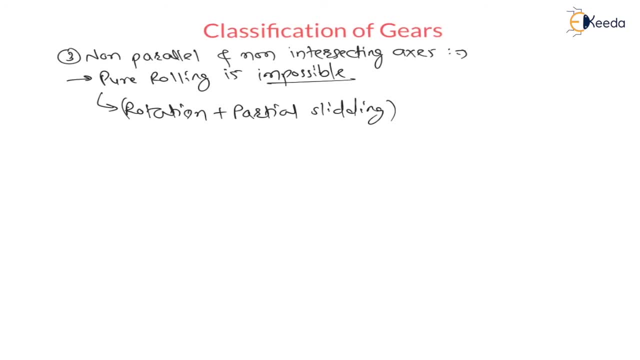 partial sliding, or translation is also: yes, rolling is possible. rotation means rolling. rolling is possible, but there is a partial sliding also, My dear students, there is a partial sliding. not slipping, it is not sleeping, it is not equivalent to sleeping, it is only partial sliding. right, therefore, in case of axis, non-parallel and non-intercepting axes. 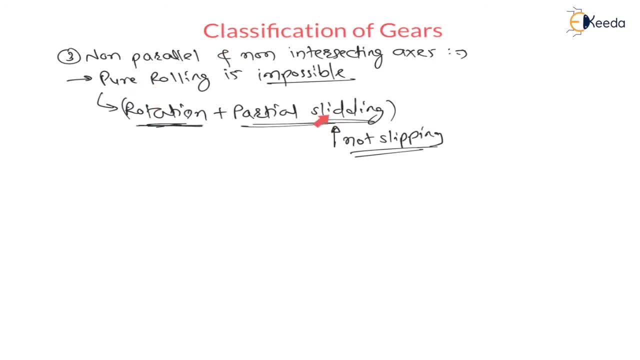 pure rolling is impossible. there is partial sliding also with rolling, for example, spiral gears, for example spiral gears. these are also called cubial gears. spiral gears are called cubial gear right, such as, for example, hypoid gear. hypoid gear, therefore hypoid gear, is an example of. 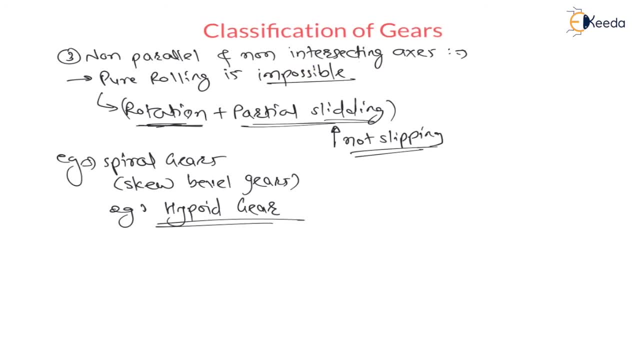 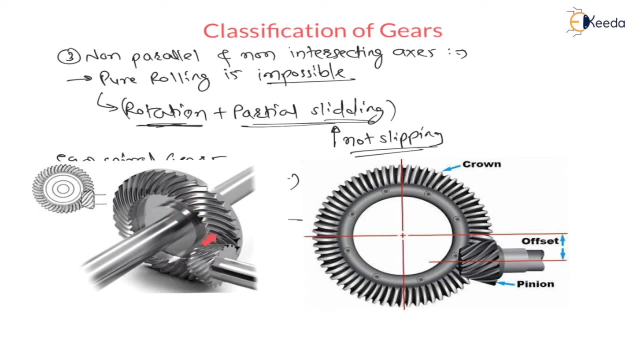 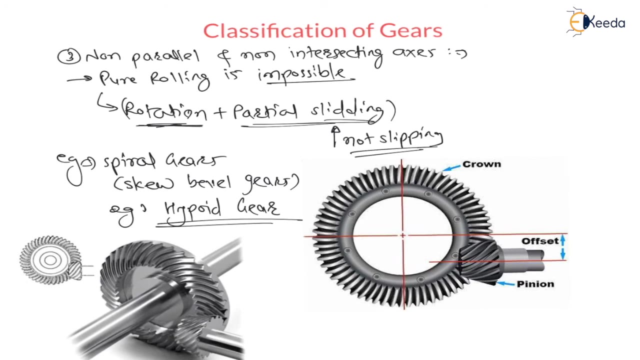 non-parallel and non-intercepting axes. now here you can see hypoid gear. see, this is a pinion and this is a gear and the power is transmitted like this. it is also called this gear is also called cubial gear or spiral gear, cubial gear. 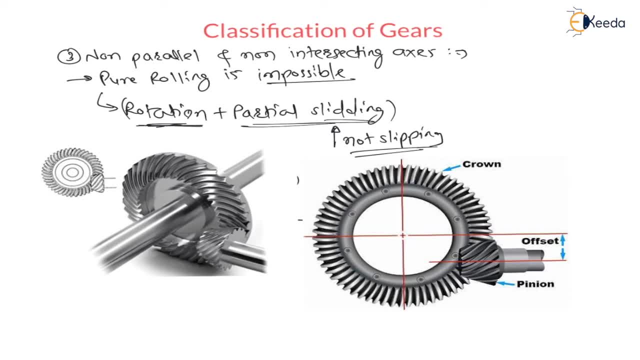 or spiral gear. now see axis. the axis of pinion is like this and axis of gear will be like this. my dear students, in this 3d view you are imagining that axes are intersected, but not because this axes are intersected. axis of pinion is passing below this axis, right in here, inside view. you can see in another view. 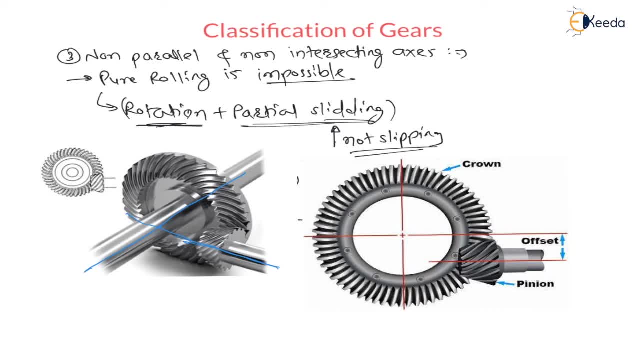 here we can see the axis is here for gear. the axis is here inward. it is going in your mobile from this point. right, it is going in mobile from this point. and axis of pinion is here. this is axis of pinion, means between axis is see here. angle between them is 90 degree, but they are. 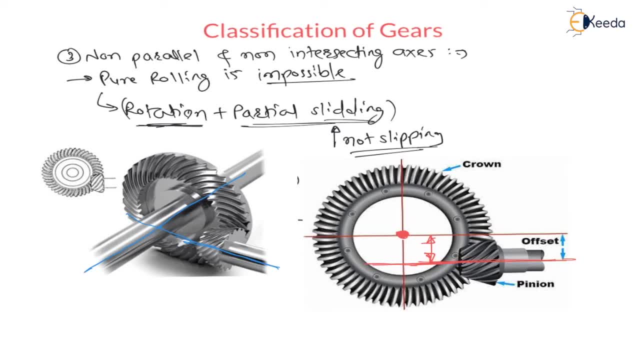 not intersecting. angle between them is 90 degree, but they are not intersecting. there is a offset. there is offset provided between pinion and gear, which is nothing but crown. the gear is called crown, remember this right. and this is non-parallel and non-intersecting axis. now the another example. 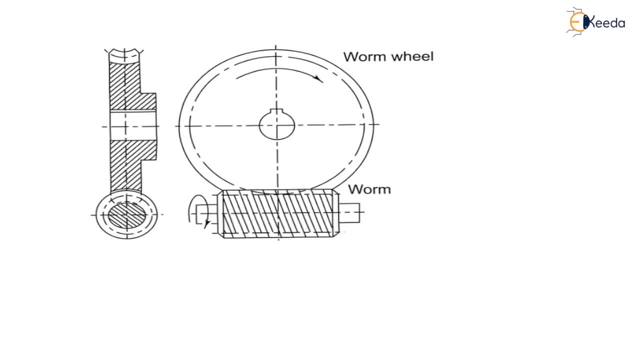 of axis are non-parallel and non-intersecting. is that warm and warm wheel? we can say: warm and warm wheel now here. you can see here warm which is rotating like this, rotation also provided. and you can see warm wheel here, warm wheel which is also rotating. now here the axis is perpendicular, see axis of warm is here and axis 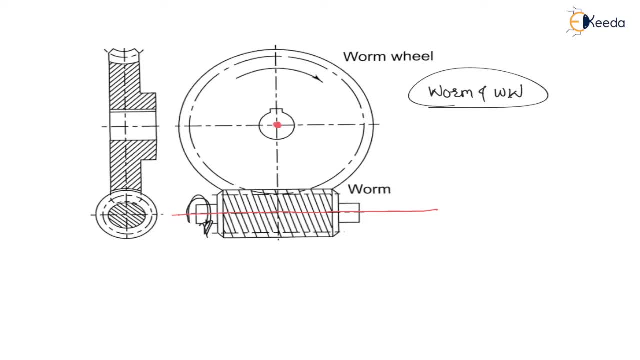 of, will be here and going inside your mobile or your laptop or your iPad, whatever may be the device you are using to watch this lecture, going inside this device, and here this is horizontal on the device. therefore, that is here we can say: it is a z-axis, it is x-axis, right? therefore, the 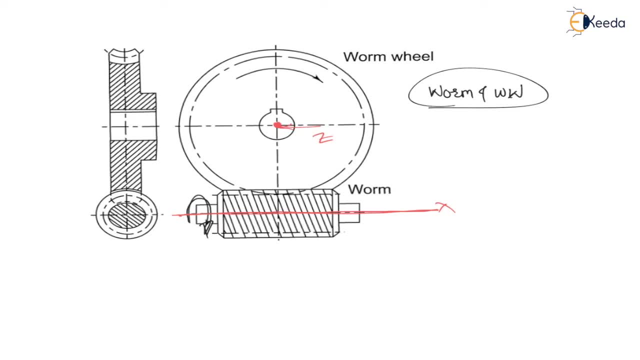 axis are perpendicular but not intersecting here. axes are not intersecting right now. generally, generally, warm is a threaded screw here. warm is a threaded screw right. and this warm and warm wheel is famous for very high speed reduction generally. its purpose is speed reduction, right, that is speed reduction, or we can say speed reduction, right. so this is the speed reduction. 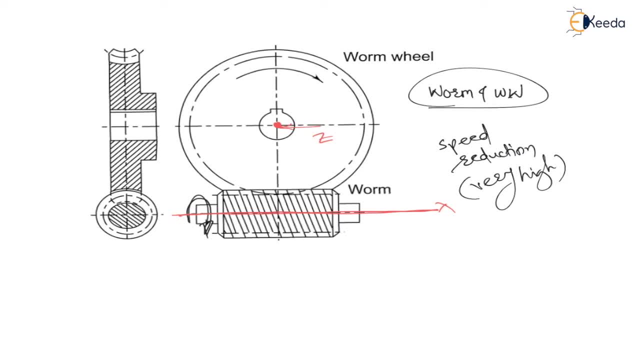 can say very high speed reduction. it is very much famous for very high speed reduction, such as, for example, it is used in guitar tightening. you might have seen guitar while playing guitar right now. if i want to tighten the guitar strings, then this mechanism- warm and warm wheel- is used also. you 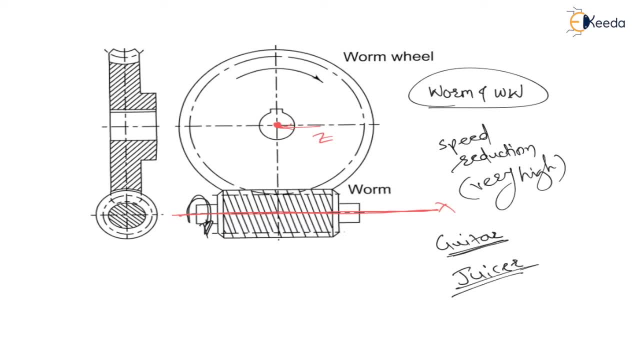 might have seen this in juicer right. this warm and warm wheel, this mechanism you will find in juicers right and it is very much famous for very high speed reduction. now, among all the gears, or among all the gear drives, warm and warm wheel provides maximum speed reduction. this is very important. my 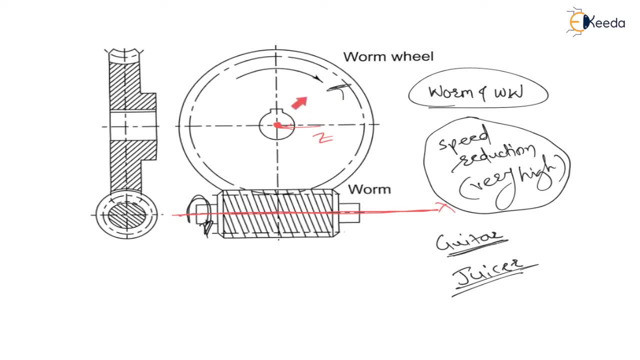 dear students. and this warm wheel imposes high radial load on the shaft right. this is also important point. in case of warm wheel, there is high radial load on the shafts. now in case of warm and warm wheel, we can say the plane of rotation is different. see, 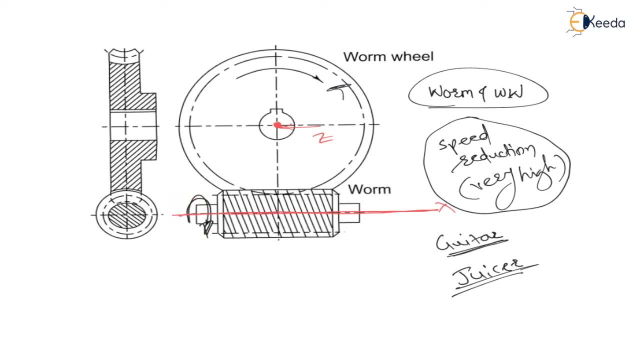 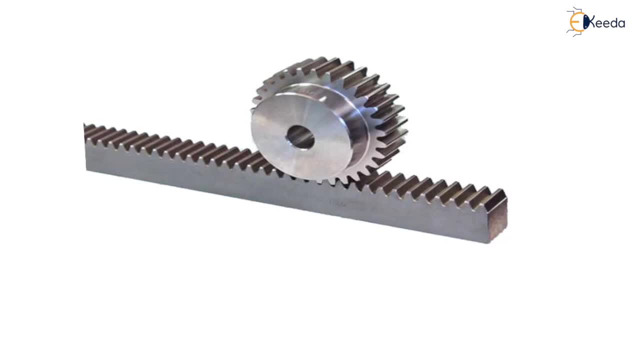 here. in this case, warm is rotating about x axis and wheel is rotating about z axis. right. the plane of rotation is different. again, very famous arrangement is that rack and pinion. rack and pinion arrangement, my dear students. pinion means having lesser diameter. now see here, this is a rack, this is a rack, that is gear with infinite diameter. we can say: 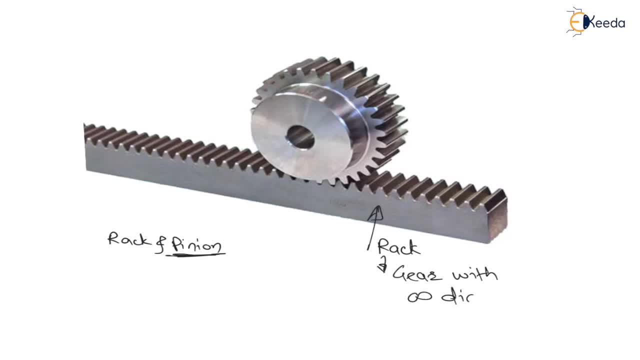 gear with infinite diameter means, as it is having infinite diameter. there is no rotation, there is only linear motion. the rack is moving only linearly right. there is only translation motion for the rack and, my dear students, the pinion is rotating. this pinion is rotating here, it is a 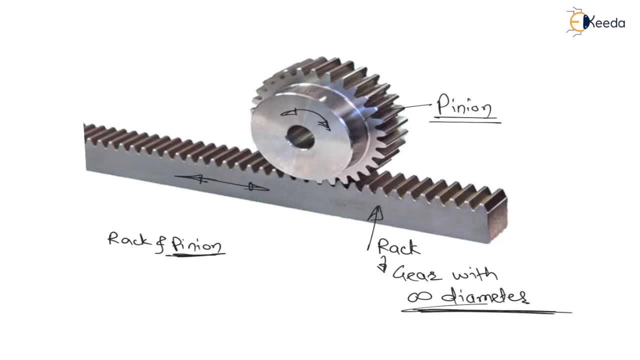 pinion. right pinion is rotating. now let us consider if i assume, let us say, the pinion is rotating in clockwise direction. let us say this is my assumption for the pinion. if pinion is rotating like this, then rack will go towards left. this will be the motion of rack. 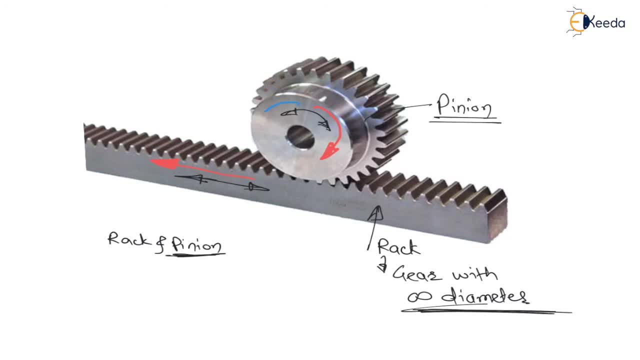 and if pinion is rotating in anti-clockwise direction like this, then rack will go towards right. this will be motion. right means in case of rack and pinion, the translation is transferred to linear motion. oh sorry, rotation. here the rack is moving in translation translation that is linear motion and pinion is rotation under rotation. therefore, 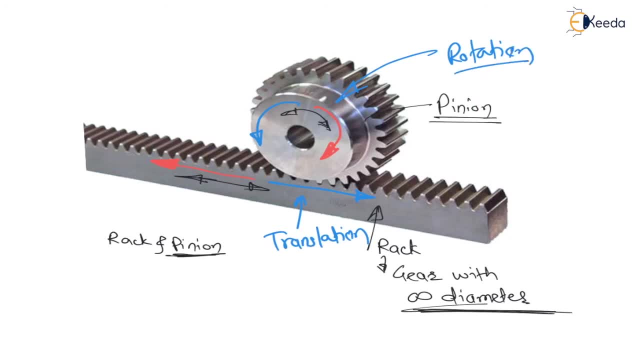 whenever i want to transfer translation into rotation or rotation into translation, then rack and pinion assembly is used and here pinion is rotating and rack is having translational motion, because the larger is called gear, smaller is called pinion and the larger one is a rack of. 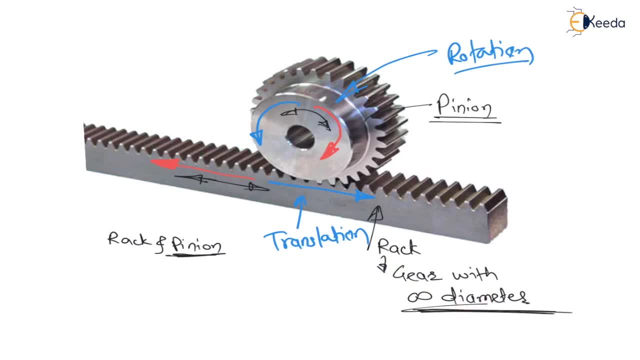 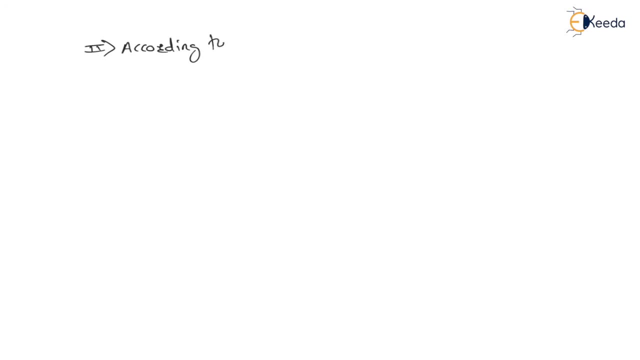 infinite diameter. rack is a gear with infinite diameter. now the second classification is according to type of gearing. according to type of gearing: in first classification we have seen according to axis of shaft. in second classification, we will see according to type of gearing. now, basically, there are two types, that is external gearing, external gearing and other is 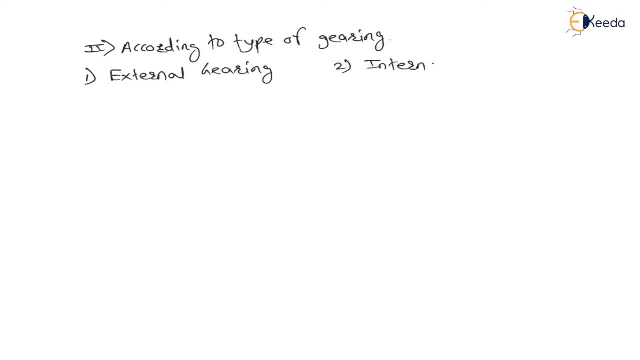 internal gearing. gearing second is internal gearing. now, whenever contact is externally, then it is called external gearing. let us say it is a gear. now there is a pinion, right, the larger is called gear and the smaller is called pinion. and if i see the another view, another view, the gear will be. 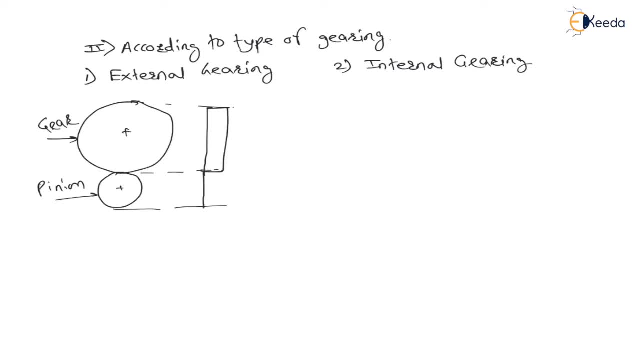 having some thickness. let us say: this is the gear and it is a pinion. they are in contact in mesh. this is the axis of gear and pinion. let us say it may be a spur gear or it may be a helical gear or any other arrangement. now here for external gearing, if gear rotates in clockwise direction. 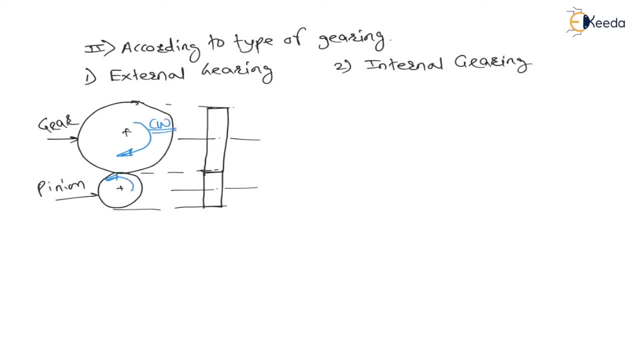 see this is a clockwise rotation for gear. then pinion will rotate in anti-clockwise direction. right means there is a opposite rotation. for external gearing there will be opposite rotation because the common contacting point will move in same direction. because of this, there will be a opposite rotation right, and this is how side view is shown, or? 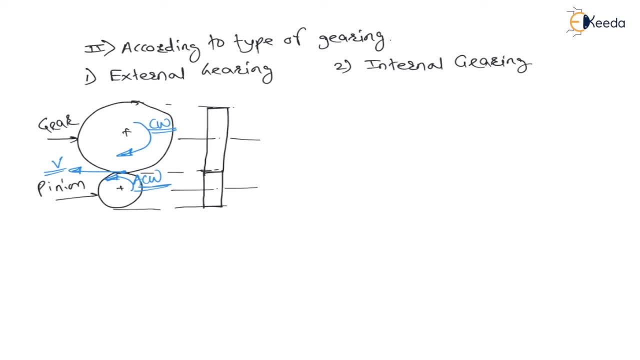 represented now. second type is internal gearing. now for internal gearing, one gear is, let us say, the larger, one is called here ring or annular, and the smaller inside. this is pinion. let us say: this is the center of larger and this is the center of smaller. now the side view is represented like this: 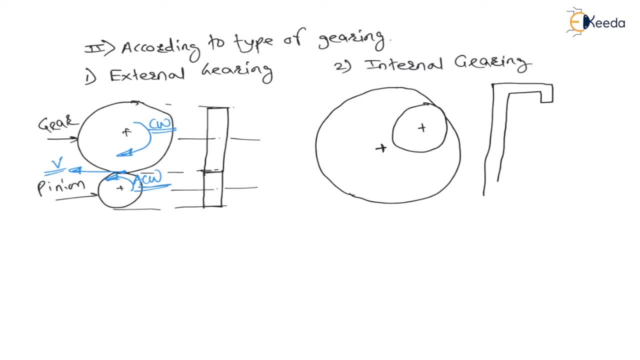 the larger. larger is shown like this: this is a larger and this is the axis of larger, and smaller is represented like this and this is the axis of smaller right. and here, in case of internal gearing, smaller is called pinion, always smaller is pinion. and in case of internal gearing, the larger or bigger is called annular or it is also called 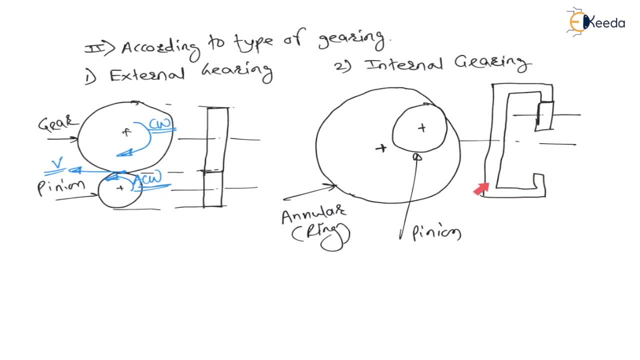 ring. it is also called ring and the side you represented is like this, like this: if such type of arrangement you will see in exam, then it is a internal gearing. and if such type of arrangement you will see, then it is a external gearing. and, my dear students, for internal gearing, 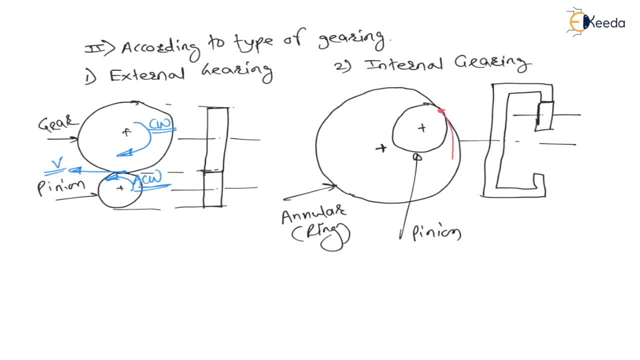 the common contacting point will move in same direction. therefore, whenever gear, annular or ring is rotating in clockwise, then pinion is also rotating in clockwise means. here the rotation is same. for internal gearing the rotation is in same direction. for external gearing the rotation is in opposite direction. now again, if more than one gear is mounted on same shaft, it is called compound. 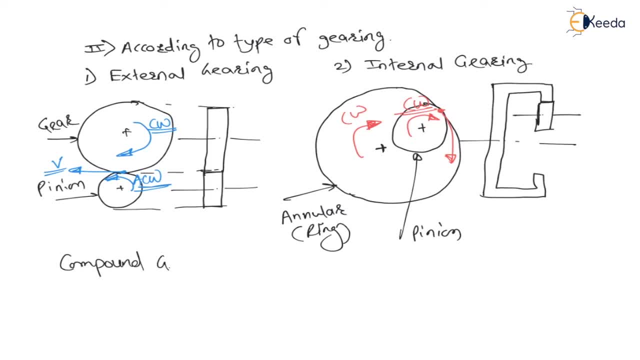 gear, compound gear means on one shaft, on one shaft, more gears, more gears, right, and that you are going to see in theory of machine topic, that is, gear train. in gear train you will learn this compound gearing. there is a simple gear train, compound gear train, right. this is the epicyclic gear train, right. these. 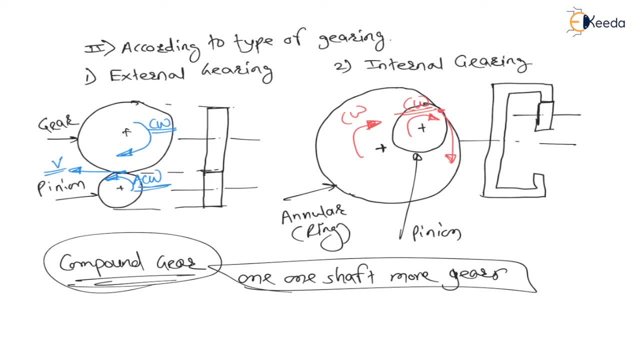 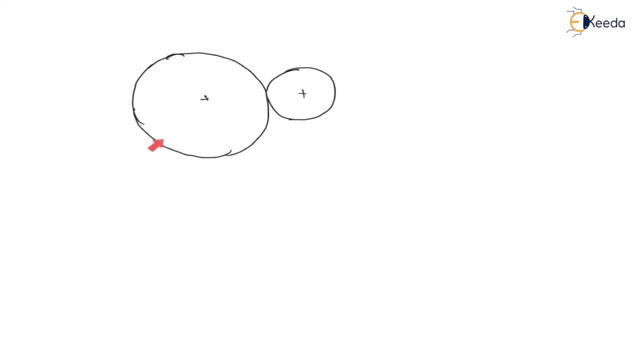 all gear trains. you are going to learn in theory of machine topic, right? if on one shaft many gears are used, then it is called compound gearing. now, during power transmission, the smaller gears are made as drivers. let us say: this is smaller which is pinion, and larger which is gear. now, during: 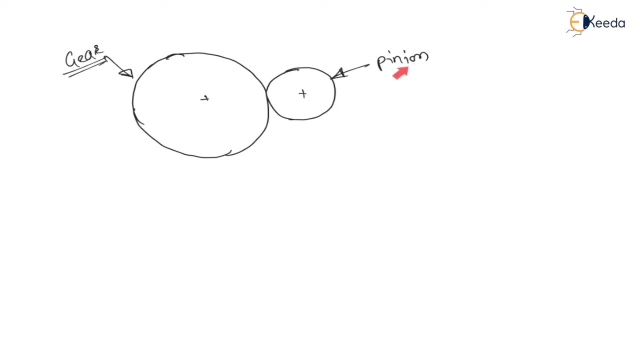 power transmission. transmission, the generally pinion, is made as driver, because power is nothing, but power is nothing but torque into angular velocity. into angular velocity. right now, see, let us say, for larger gear radius is r1 and angular velocity is omega 1, for smaller gear, radius is r2 and angular 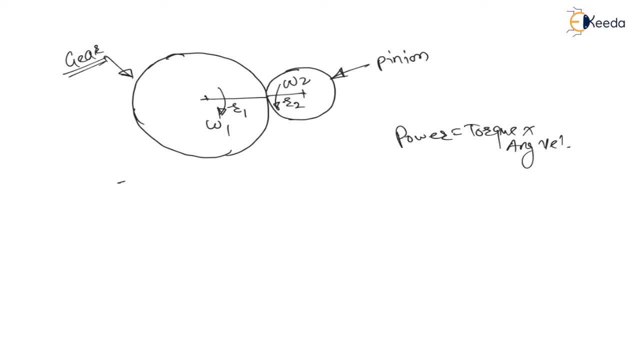 velocity is omega 2 and already we have seen that r1 omega 1 is equal to r2 omega 2. now, as r1 is more than r2, then omega 1 must be less than omega 2. right means larger gear. having larger, smaller gear is having more angular velocity. angular velocity is more for smaller. 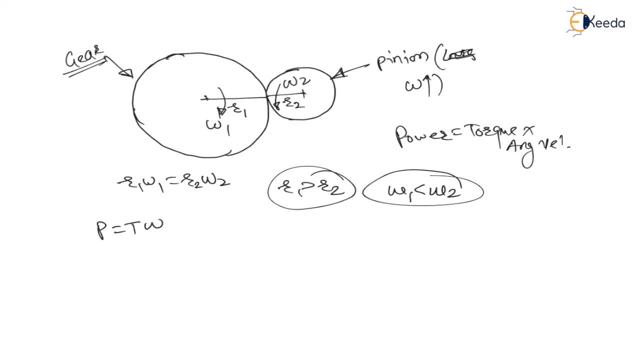 gear right and power is nothing but torque into angular velocity. therefore, if angular velocity increases, then torque required decreases. right now, torque required is nothing but input. torque required is nothing but input. therefore, for power transmission generally, pinion or smaller gear is made as a driver so that the input torque required to drive the gear is less or minimum. right now. 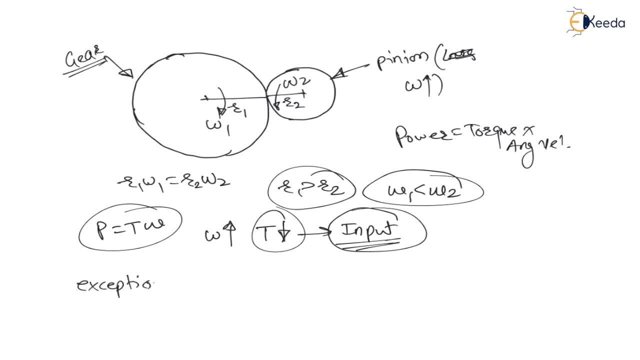 exception is there for every case. there is always exception. exception is that bicycle, bicycle, my dear students. in case of bicycle, the power is given, or torque is given to the larger, because to minimize the pedal rotation or to minimize human fatigue, right, if power is. see who is giving power in bike. in case of bicycle, your legs are giving power to the pedal. 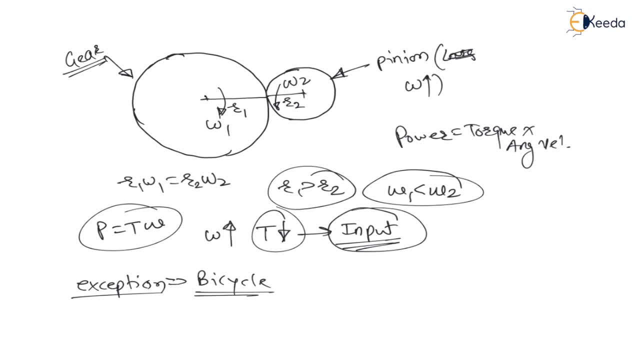 a pedal is rotating at larger radius. pedal is rotating at larger radius. why? Because if pedal is rotating at minimum radius, then as number of rotation increases, then your pedal movement also increases. Because of this, in case of bicycle, to decrease human fatigue, only the power is given or the torque is given to the bigger one. 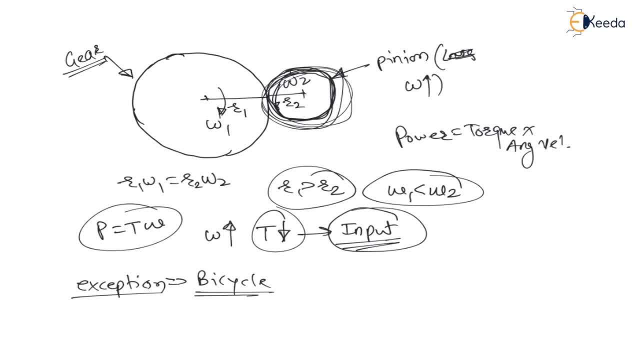 But if torque is given to the smaller one, lesser torque is required. Now observe any vehicle. The vehicle having bigger pedal requires more effort to run, And vehicles with very small pedal requires very small force or very small torque to run. Now the selection of gears depends on the various parameters. 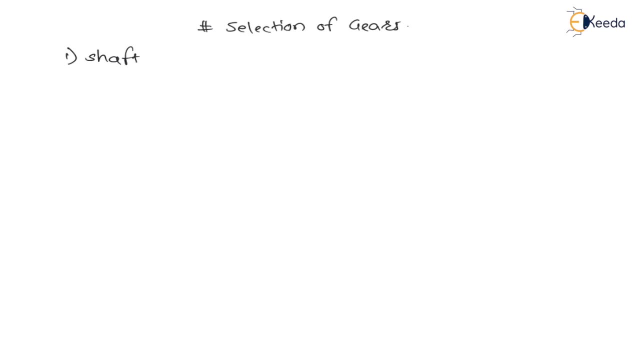 Let us say first is if shafts are parallel, then we have two types, That is, we can use spur gear Or we can use helical gear. Now, spur gear is cheaper And helical gear is little bit costlier. 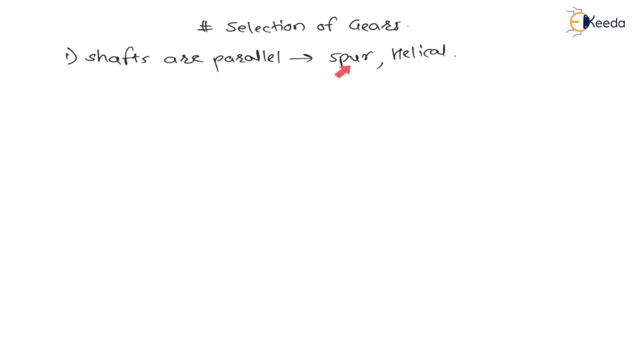 But in case of spur gear, due to sudden engagement and disengagement, there are impact stresses And in case of helical gear, this problem is eliminated. There is a gradual engagement. Therefore, there is no impact stresses. that already we have discussed. 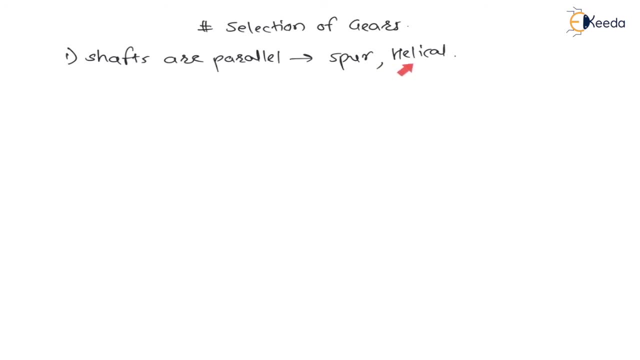 Now, therefore, for high speed power transmission with parallel shafts, helical gears are used Right. And again for velocity ratio. Velocity ratio up to 6 is to 1. Then we can use spur gear or helical gear. 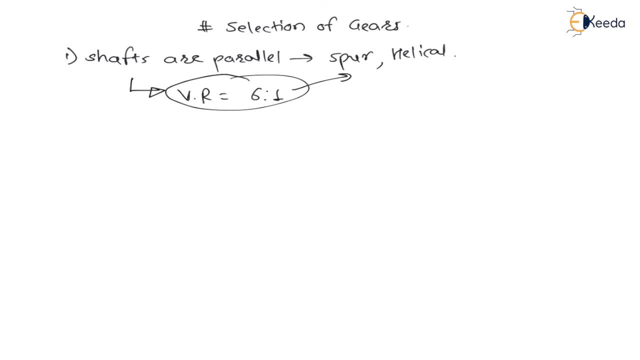 Right. Whenever velocity ratio is 6 is to 1, then generally spur and helical gears are used, Which may be extended up to 10 is to 1 also, But in rare cases. generally it is 6 is to 1.. 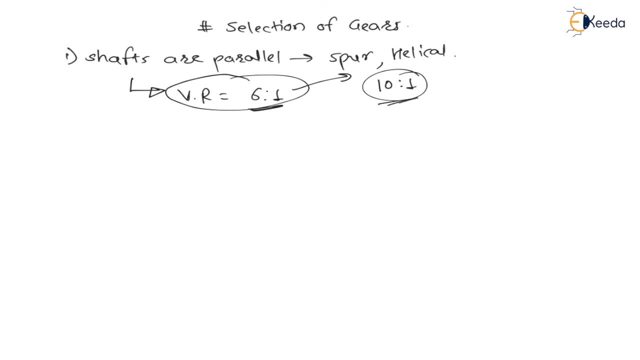 In rare cases we can extend this velocity ratio up to 10 is to 1. Right Now. the second is when shafts are intersecting. Shafts are intersecting at 90 degree. Then we have bevel gears. 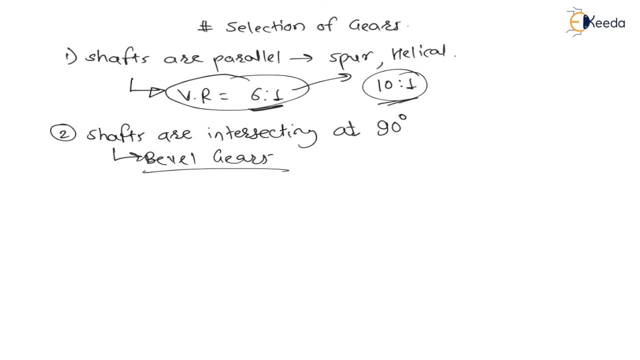 Then we have bevel gears. Bevel gears are used whenever shafts are intersecting and at 90 degree The shafts. the intersection is 90 degree or sometimes less than 90, or more than 90 is also preferred Right. 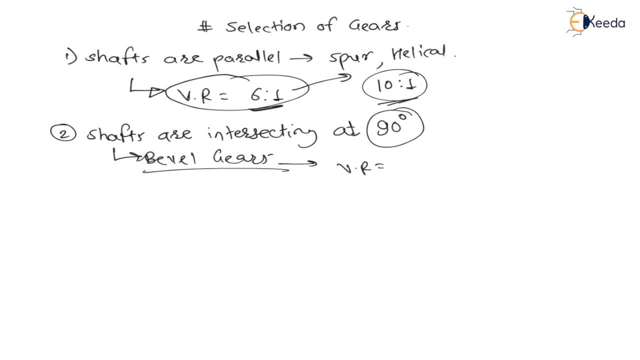 But in case of bevel gear the velocity ratio is 1 is to 1. Means velocity ratio is very small Means. here only power is transmitted at 90 degree. But up to some extent velocity ratio can be increased. up to 3 is to 1, also in case of bevel gear. 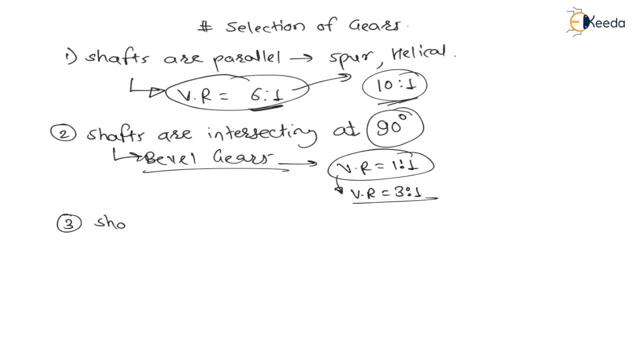 Third point need to be considered is when your shafts are non-parallel, non-parallel and non-intersecting. Non-intersecting And angle between them is 90 degree. Means angle between the shafts is 90 degree, but they are not intersecting. 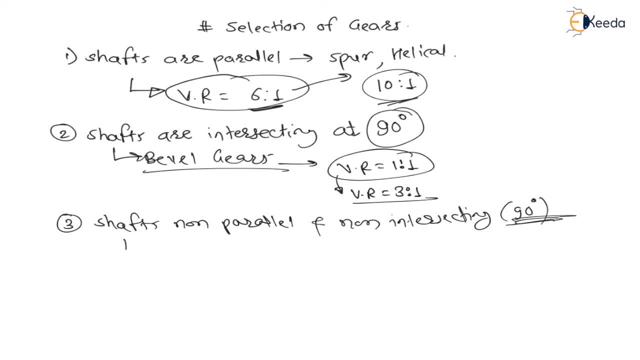 As angle is there, they are not parallel. also, Then we are using warm and warm wheel, That is, warm gear, warm and warm wheel, And for very high speed reduction, that is, velocity ratio up to 60 is to 1.. 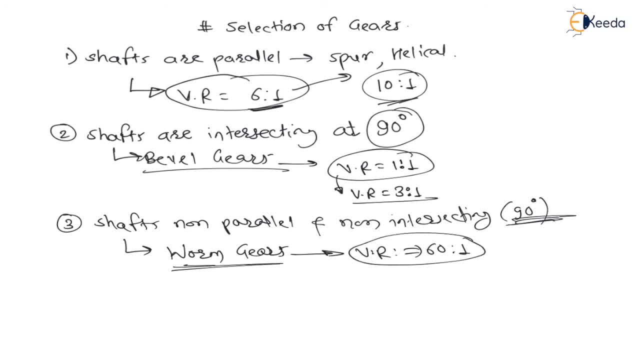 That means for very high speed reduction. we can use warm and warm wheel And up to some extent the velocity ratio can be increased. up to 100 is to 1. Means very, very high speed reduction in case of warm and warm wheel.